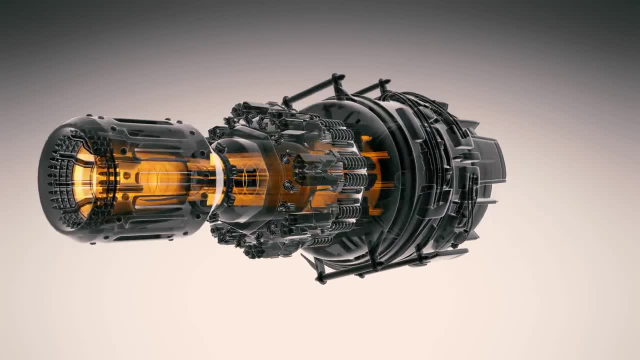 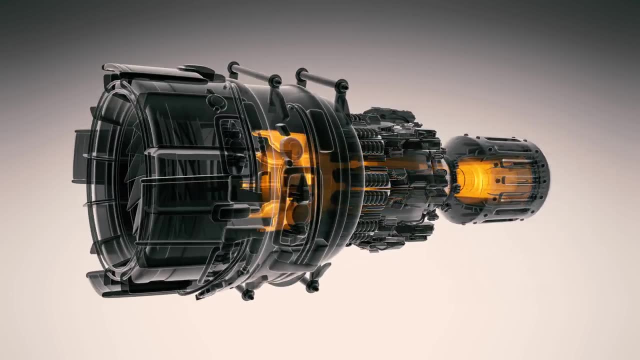 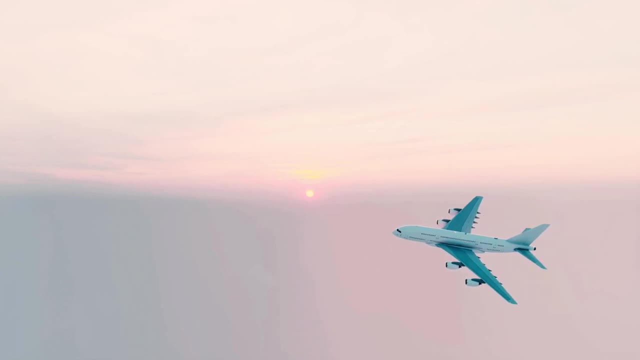 In aeronautics, the focus is primarily on understanding aerodynamics, propulsion systems, control mechanisms and materials used in aircraft construction. These experts work on optimising aircraft performance, stability and manoeuvrability to ensure smooth and safe flights for passengers and cargo. Now let's journey beyond Earth's atmosphere and see what we can do to improve. 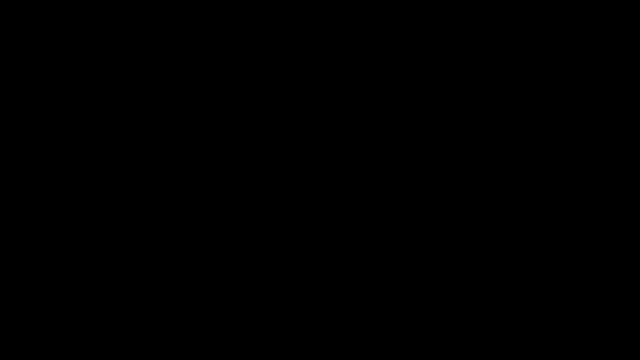 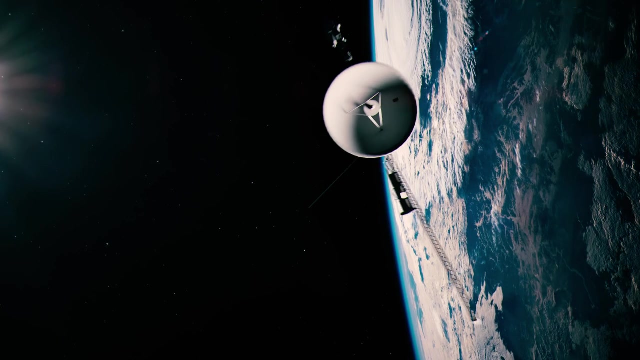 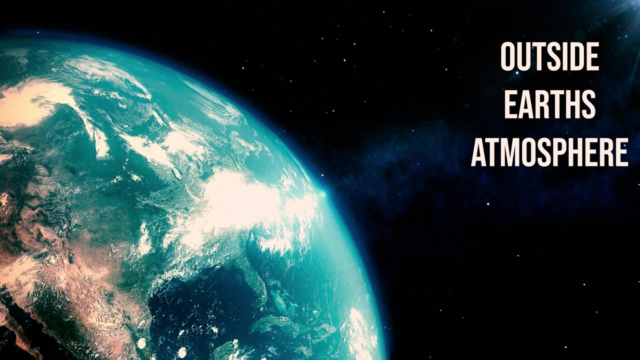 the47th Trans-Pacific Question in 06-6.. And explore the realm of Aeronautics. Aeronautics involves the science and technology of space travel and exploration. It encompasses everything related to spacecraft, rockets, satellites and the various systems and technologies. 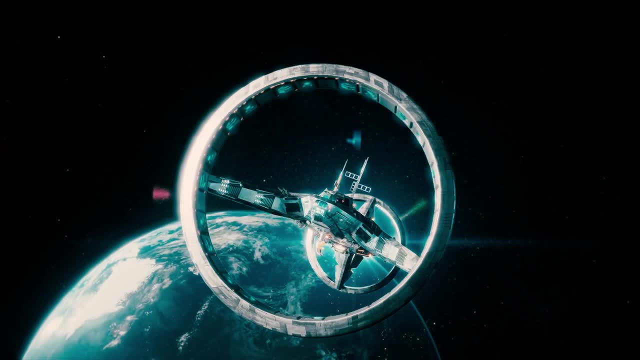 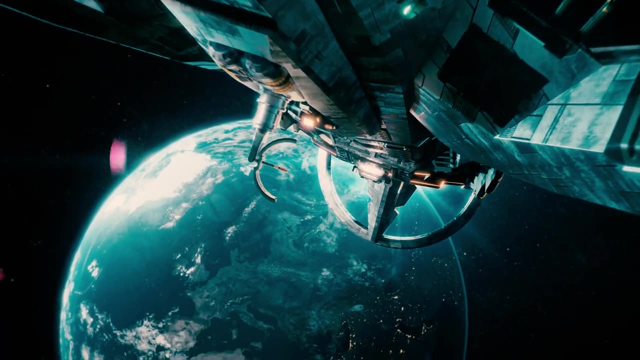 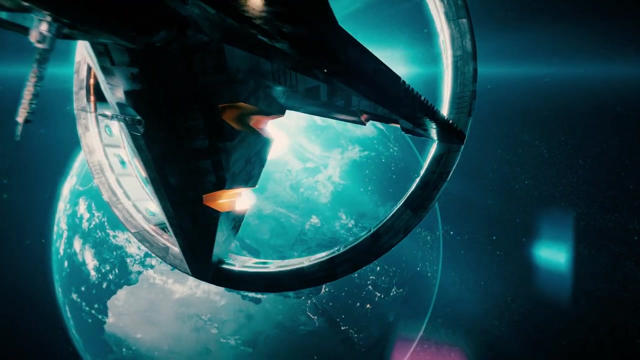 used to operate in the vacuum of space. Astronautics is all about pushing the boundaries of human exploration. Astronautical engineers focus on designing and developing space. It's about envisioning and developing space for spacecraft capable of carrying humans and payloads to destinations beyond Earth. 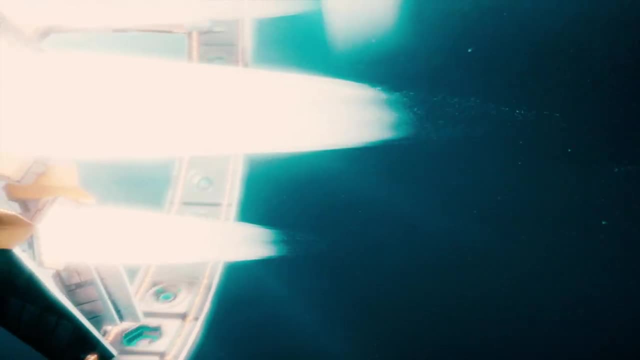 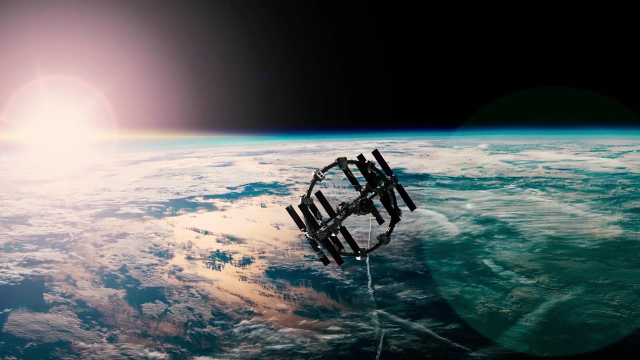 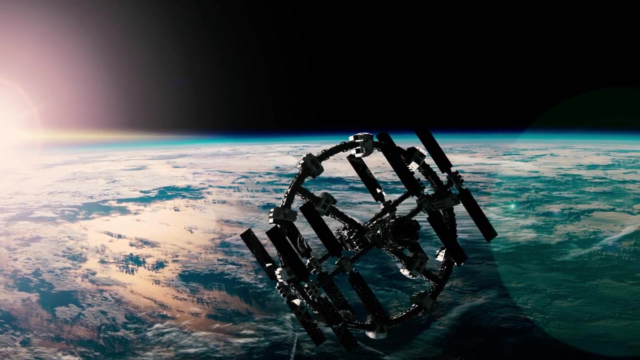 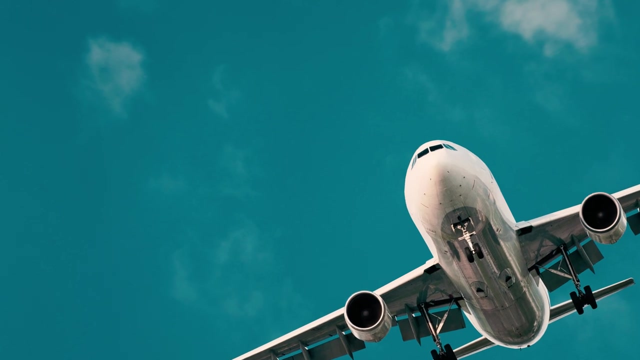 They tackle unique challenges such as escape velocities, microgravity environments, life support systems and celestial navigation. Now that we understand the basic concepts of Aeronautics and Astronautics, let's highlight some key differences between the two. Number 1, Operating Environment Aeronautics, deals with the flight within Earth's 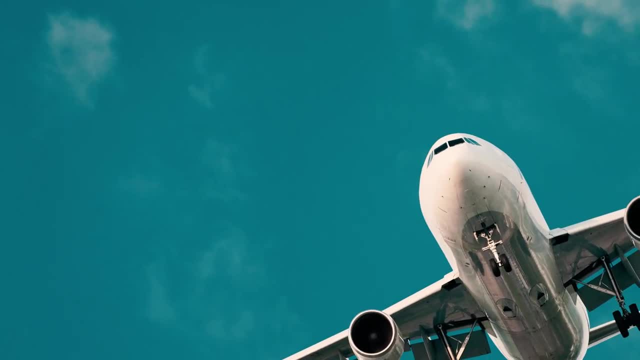 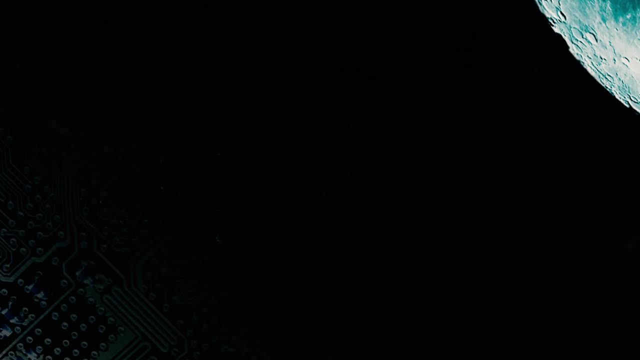 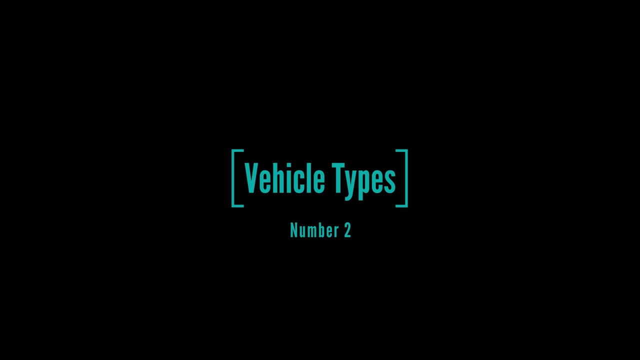 atmosphere, where the air provides lift and other aerodynamic forces. In contrast, Astronautics focuses on operating in the vacuum of space, where there is no air to generate lift or propulsion. Number 2, Vehicle Types. Aeronautics mainly deals with designing and 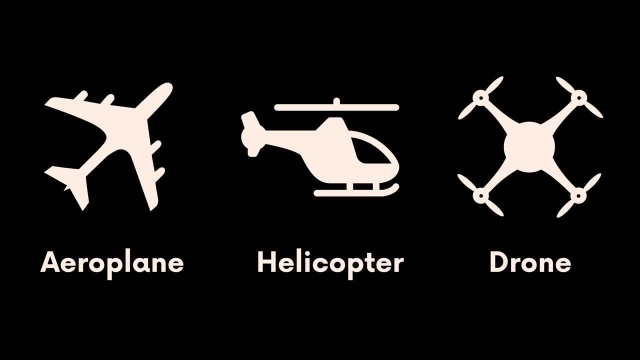 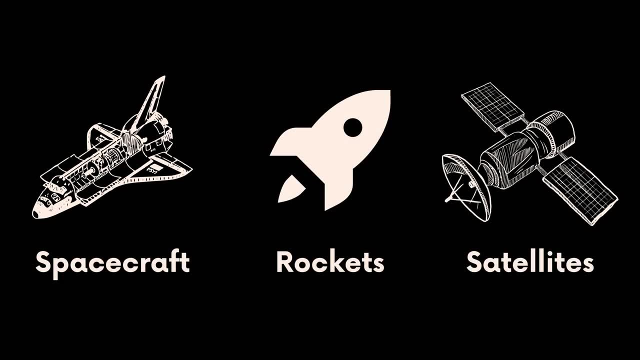 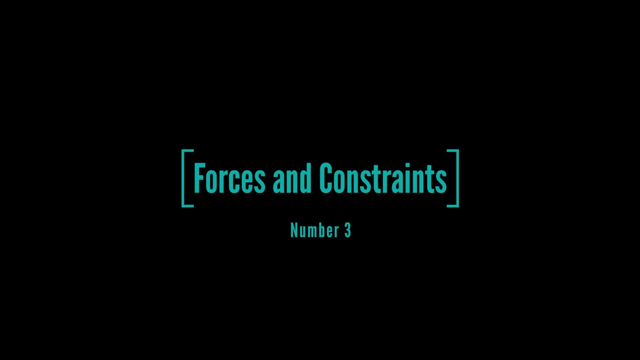 operating aircraft, including aeroplanes, helicopters, aircraft carriers, aircraft helicopters and drones. Astronautics, on the other hand, is concerned with spacecraft, rockets, satellites and space probes. Number 3, Forces and Constraints. In Aeronautics, engineers must consider gravity. 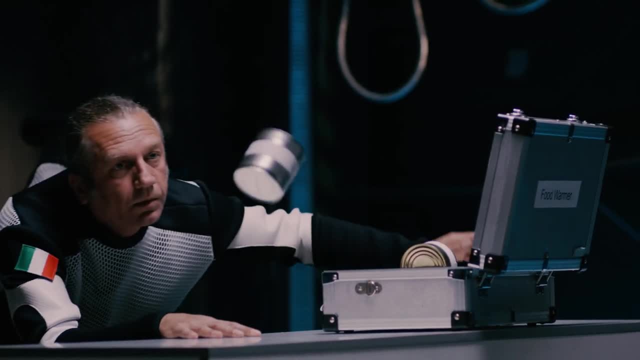 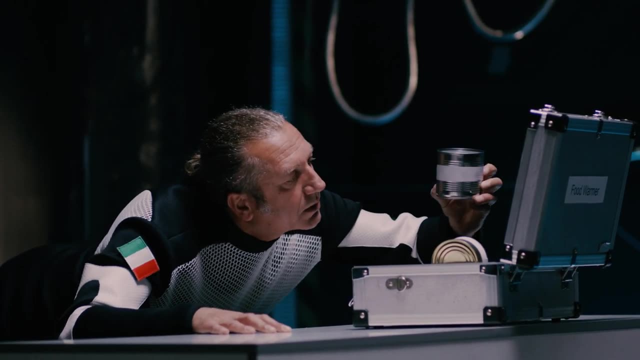 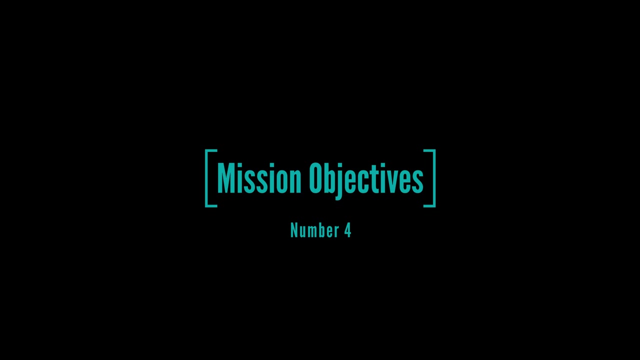 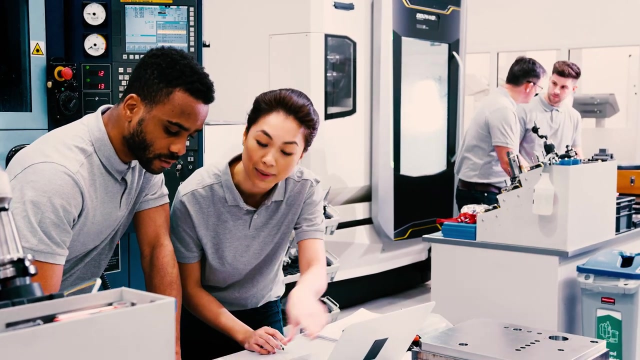 drag lift and other atmospheric conditions. In Astronautics, the primary forces to contend with are gravity, inertia and the absence of atmospheric pressure. Number 4, Mission Objectives: Aeronautical engineers work toward improving aircraft performance, passenger safety and fuel efficiency.